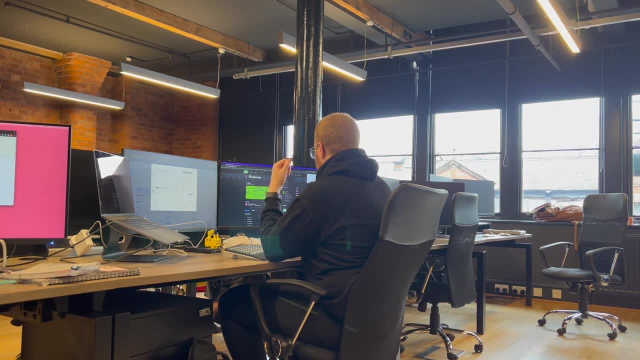 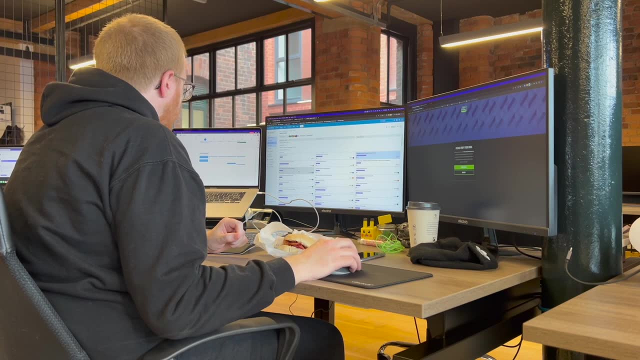 looking through my Jira boards just to see where my priorities for the day should be. If I'm working from the office, usually I'll pick up a coffee and a bacon and sausage sandwich on the way in, so I can get straight on with checking out missed emails and messages on my Jira boards once I get in the office. 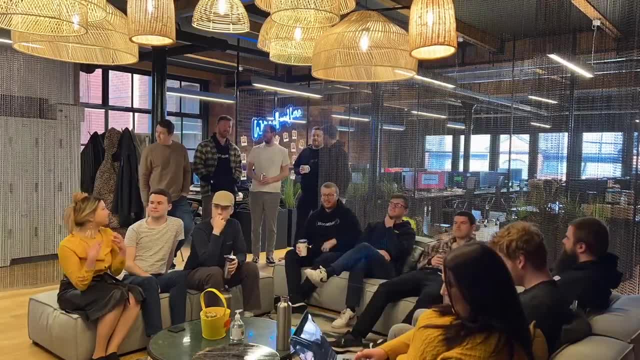 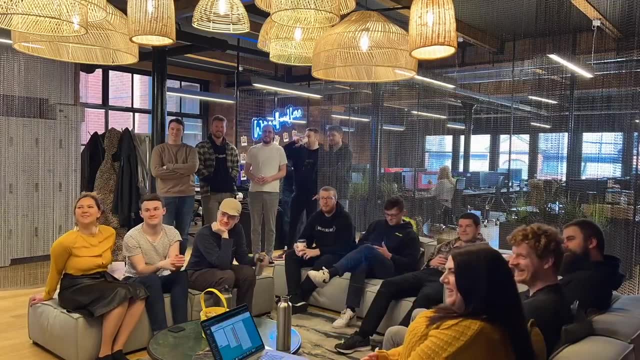 On a Monday, we have our daily stand-up meeting around about quarter past 10.. So during this meeting that's normally the perfect opportunity to find out if any of the devs on my team have any issues or any blockers that need testing after campfire. 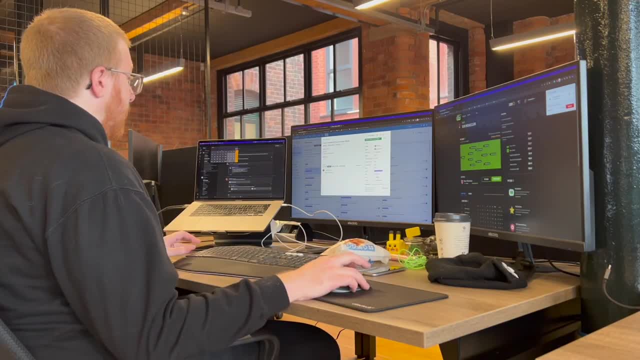 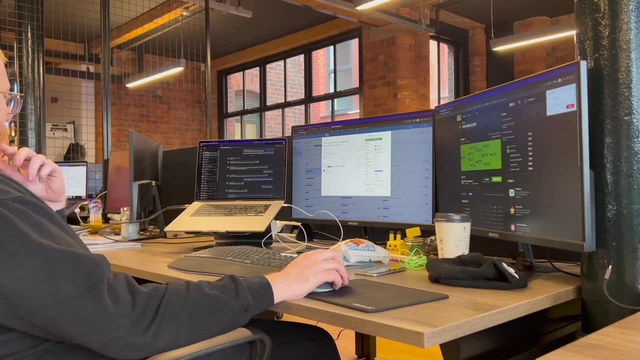 After checking through the Jira boards I work from, any urgent or high priority tickets are usually what I'll start with, since they're urgent or high priority. If there aren't any urgent or high priority tickets, it entirely depends on if there's any project deadlines coming up or not. 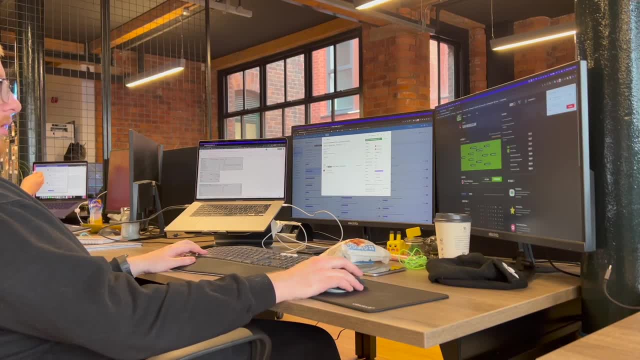 I mean, if there isn't, I'll be a case of working through any of our warranty or support tickets. Otherwise, the project works normally, while I'll always prioritise just because there'll either be a deadline for it coming up or we need to get it in for an internal demo. 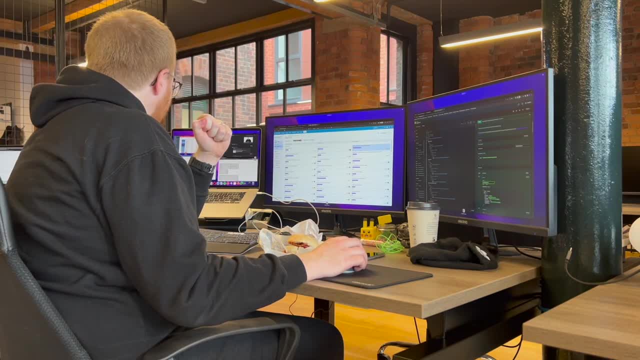 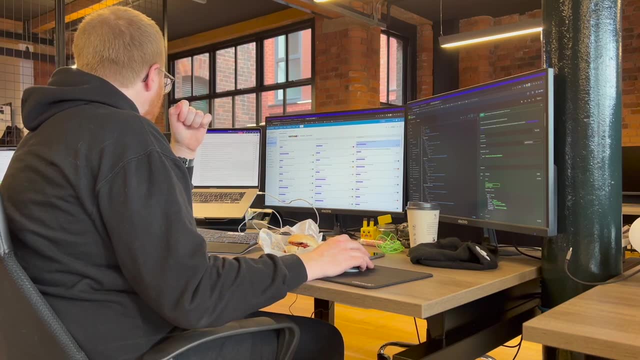 Because my important tasks tend to be the urgent or high priority tickets or project work that has upcoming deadlines, I'll usually start my day off with these. Sometimes, for bigger pieces of work, this can drift into the afternoon or even take up a full day. 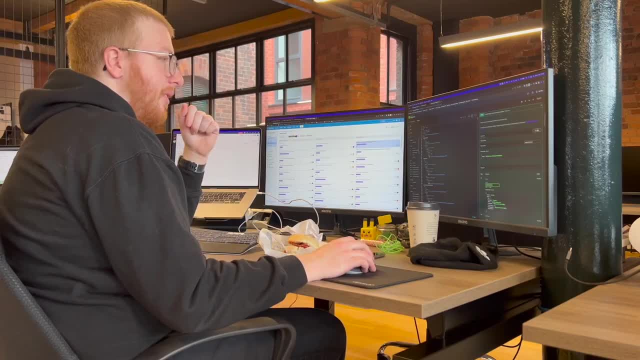 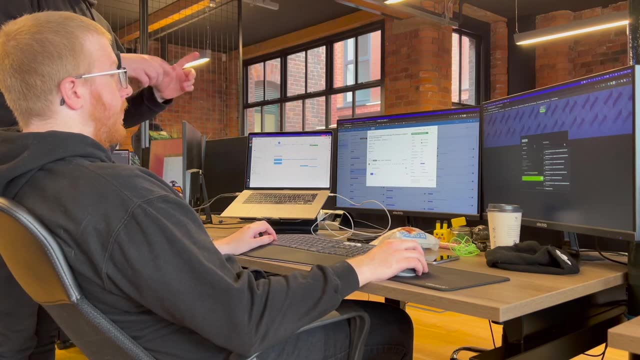 However, that only really happens with project work and there's a rarity outside of this. I mean. a standard working day usually consists of me making sure any work that the developers have completed is working as expected from the point of view of an end user for the site. 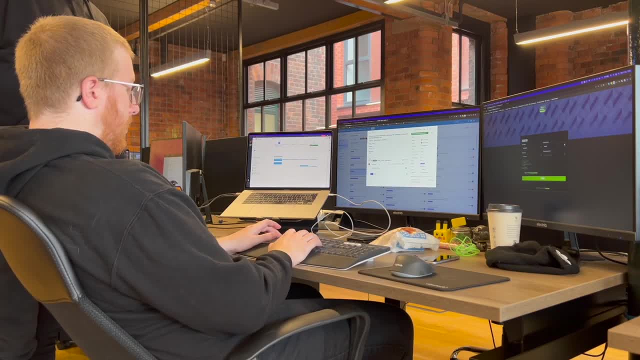 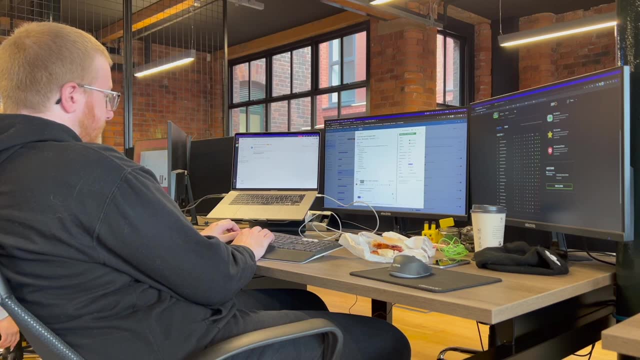 Just making sure there's no issues with the functionality, the designs or the user experience of the section of the site or app the work's been done on This. usually is done by working through a set of pre-defined acceptance criteria. if working on a support ticket. 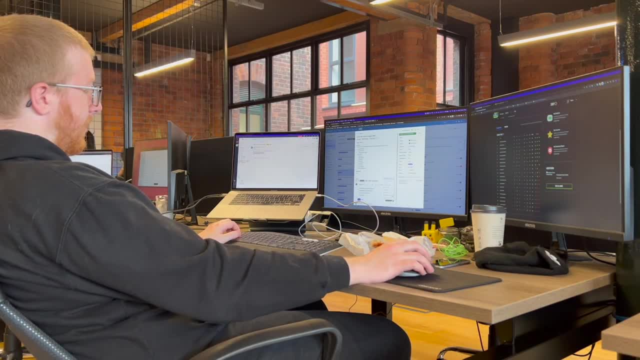 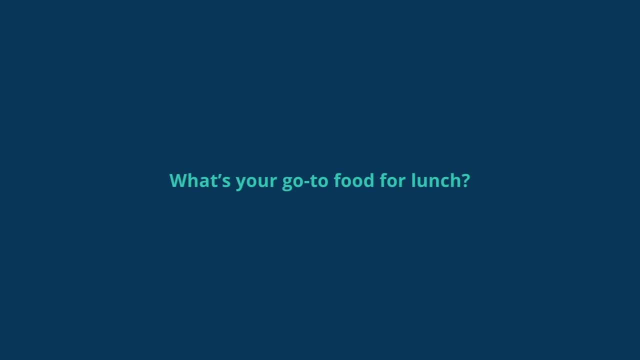 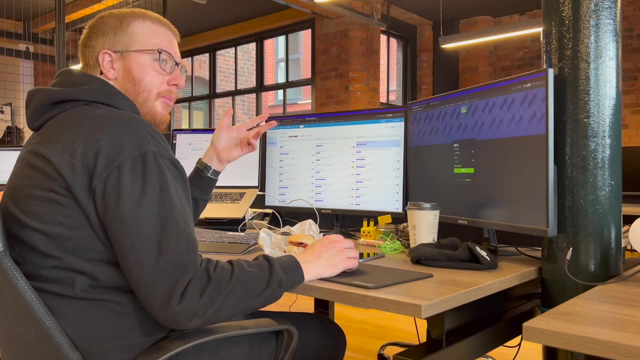 or based on the ticket description or the project specification. if working on a project or some project warranty work. Burger King's been kind of like the go-to place recently. However, you can't really beat a decent Greggs, or Roadies is also a safe second choice. 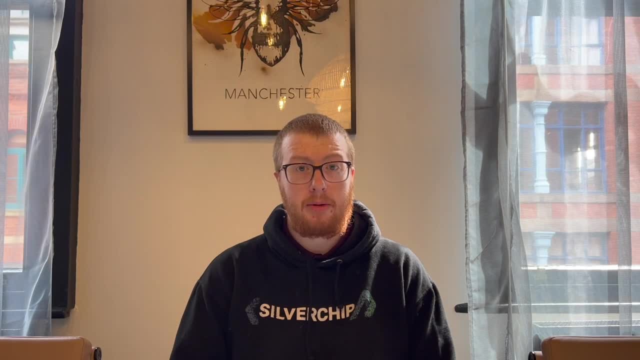 So the essential tools that I use for my job would be my laptop, the web browsers I've got installed on there so I can do some cross-browser testing. The mobile devices: we have some iPhone and my Android phone so we can test out mobile applications. 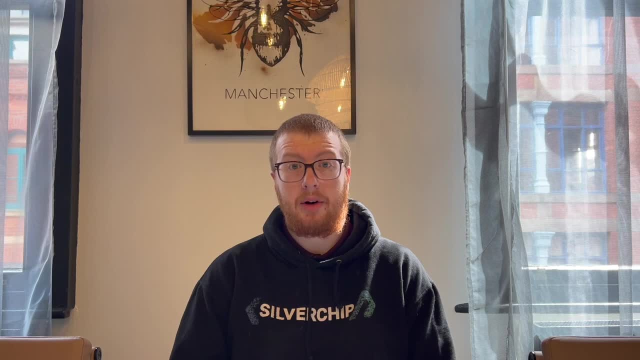 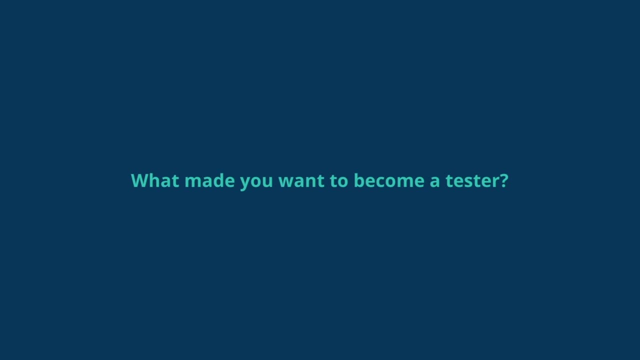 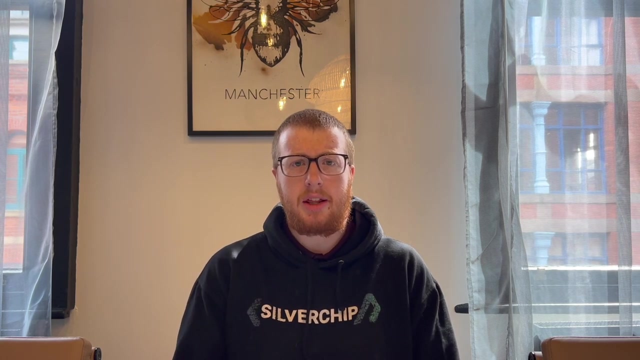 We do also have a website we use for our automated pen testing called App Check. I'm a very sort of logical and methodical person. for as long as I can remember, When I was younger, I always used to like sort of taking things apart, seeing how they worked, but kind of didn't really know how to put things back together. 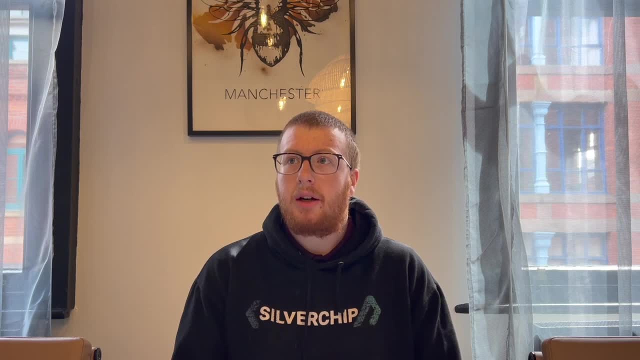 Yeah, I think all of those things put together are kind of why I enjoy testing. That kind of came very apparent when I was at university- sort of testing games for some of my friends who were also on games design course. Definitely something satisfying about finding issues in an app or even a game. 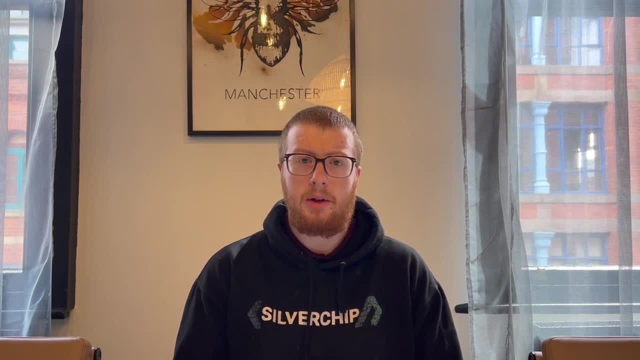 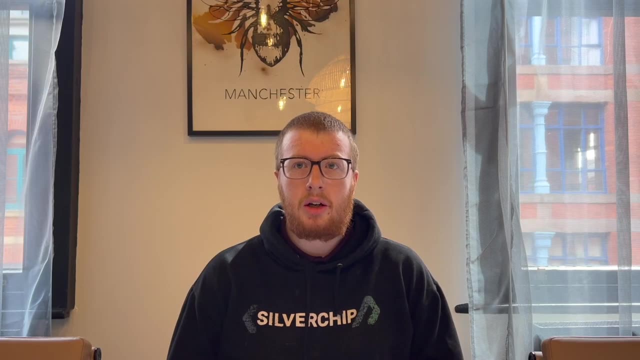 and then trying to work with people to find out what the problem was and where we can go to get it fixed. I think having a logical mindset is probably sort of the main thing. It's kind of like the core. the very good QA tester would be that. 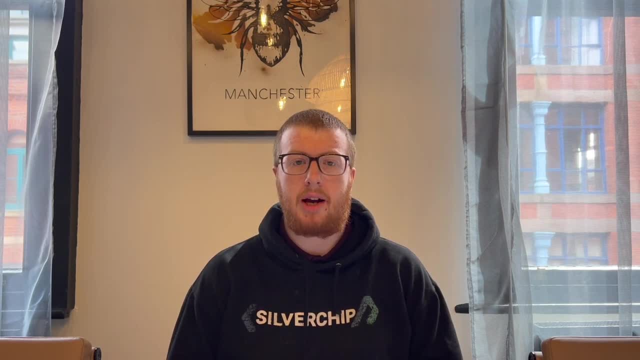 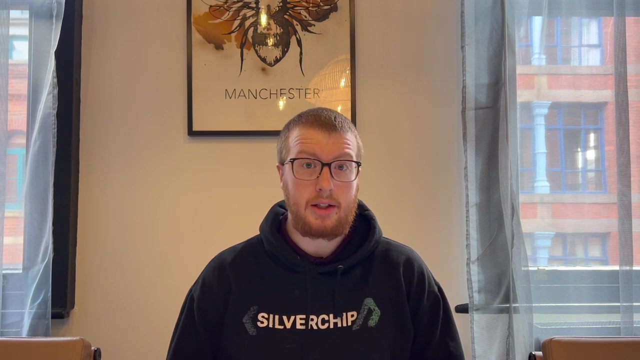 I mean following on from that. I think finding it easy to grasp new software or at least be able to understand the core concepts of that, is also kind of an important skill or a tribute to have. Beyond that, I mean being able to handle repetitive tasks, having good communication skills, getting good listening skills as well. 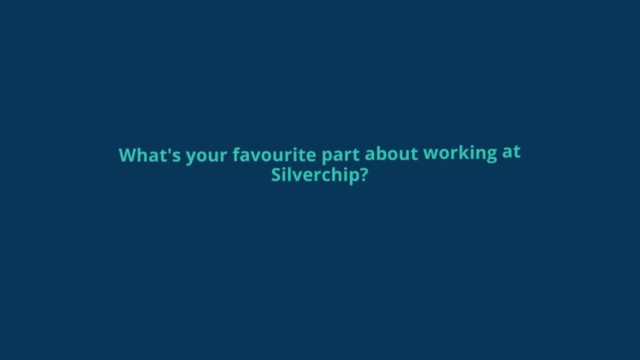 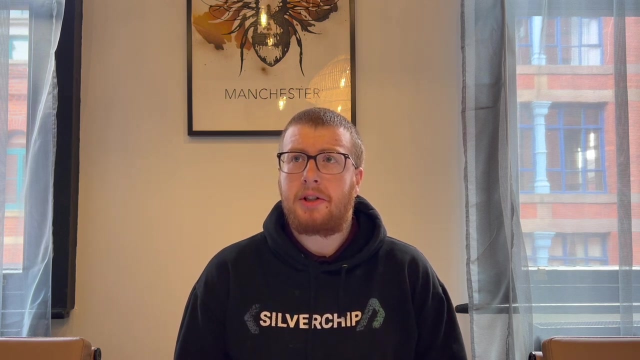 All very important things, And then when you want to be a tester, It's hard to pick one thing really. I mean, the first thing that comes to my head is a good workplace environment and probably colleagues as well, And I think when it comes to enjoying somewhere you work, those are two really important aspects. 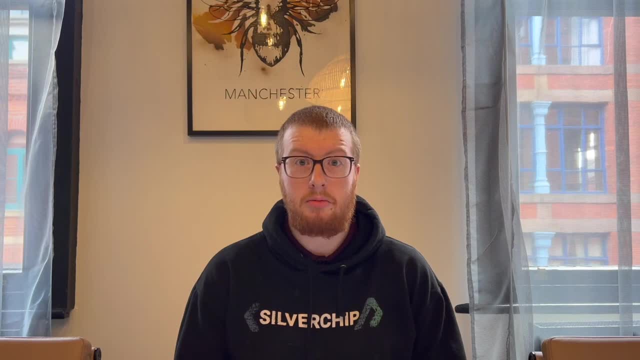 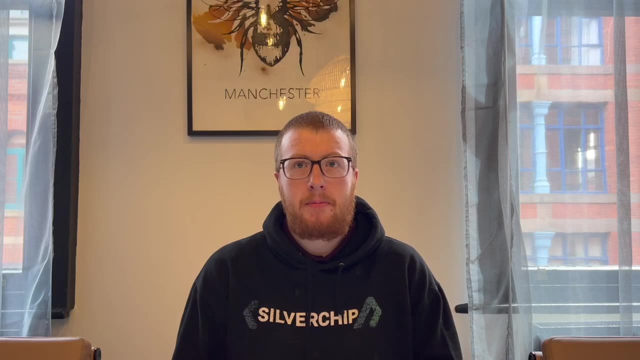 And I generally think silver chip would get both those nails on the head. It would really be a great place to work. Well, that kind of varies from day to day really. Most days I normally clear my boards between like half five and half six and I'll clock off around about that time. However, there's been times where I've clocked off as early as 4pm or as late as 8pm. Really depends how much work I've got on, how many projects I've got going on and if I need to put the extra hours in or if I've already hit my hours for the week. really. 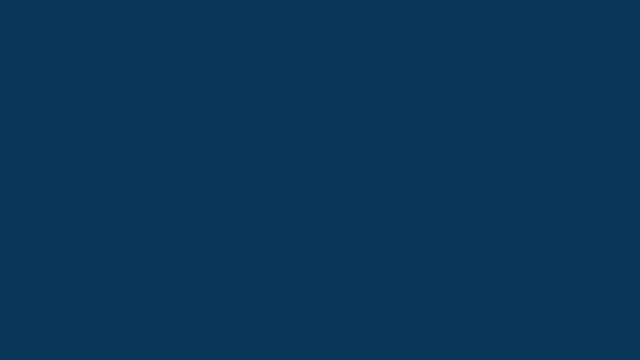 And that's my day. Thanks for watching. I'll see you next time.